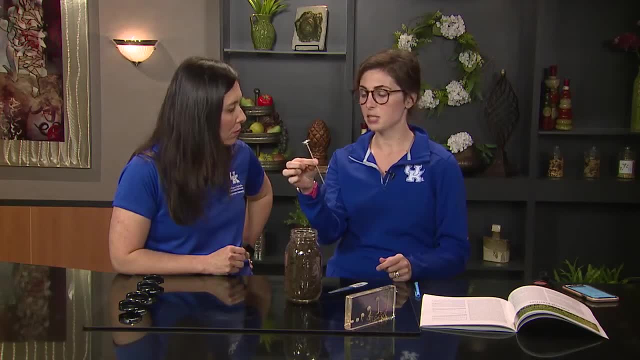 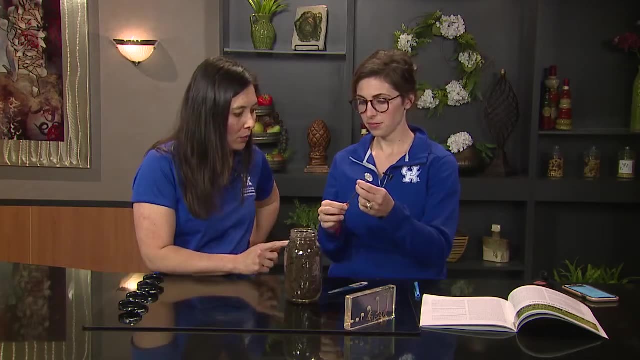 that time is pretty chilly, So when you stick this in, it's pretty important to get it at the right depth. So what depth do you think we're going to put it in? It should be an indicator on your thermometer, right? So this is one is just a little cheapo one, But you want to stick it. 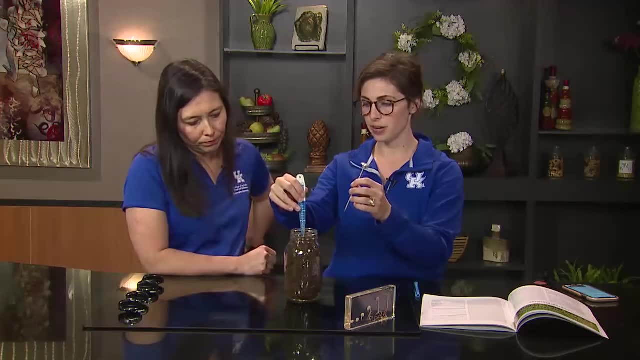 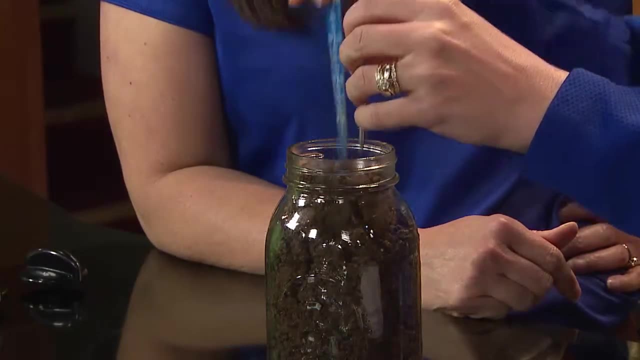 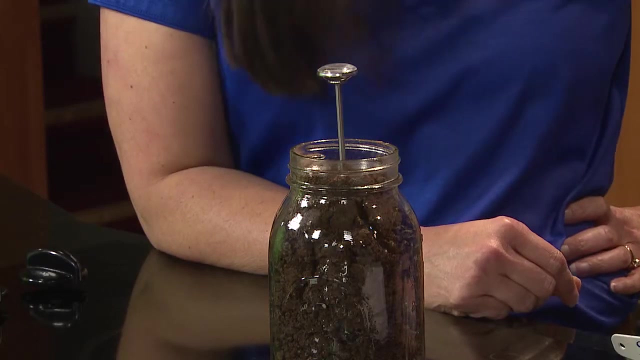 in to about your planting depth. So for soybeans we're going to go one and a half to two inches. So if you stick this in you can see about how far to go with it. So I always just kind of gauge it there, Yeah, gauge it there, and then stick it in. Now you have to wait, You can't. 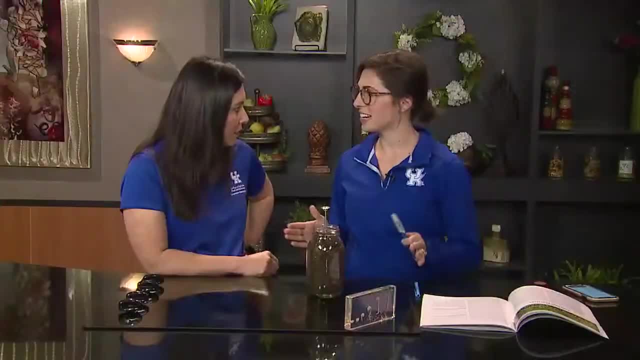 just be like: oh yep, it's 80 degrees, You have to let it kind of acclimate. So what I will usually do is stick it in, do something else and come back in about 10 minutes and double check it. So for soybeans we want about 55 degrees, For corn we can go with 50. And you want to look at your forecast for the upcoming week to see is it going to drop down really cold? Because a lot of times when you plant- and I brought this really cool diagram here- Yes, So this is your seed. 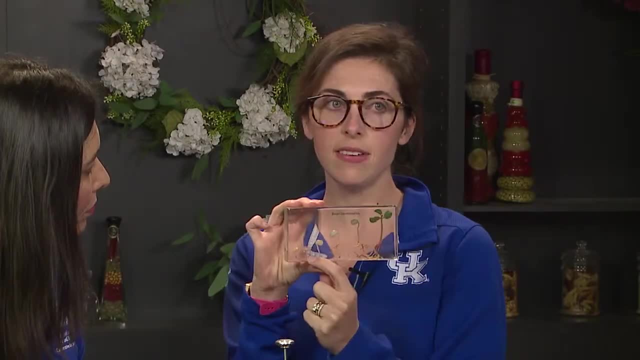 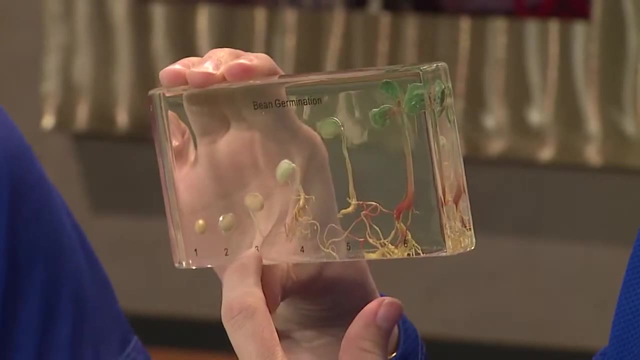 what it looks like when you're actually planting. Now it will swell, Even if it is cold out. it will swell, But from there, if the temperature is too cold, it will not sprout, It will not shoot that little root down and it will not come out. So it can swell. 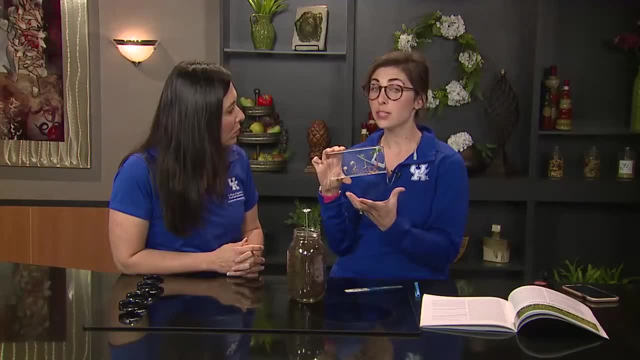 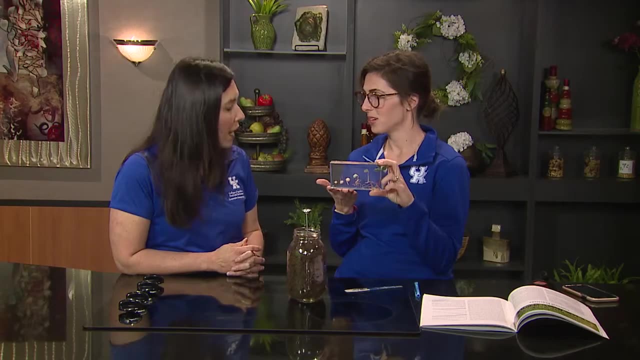 and then it will just rot if it's too cold. So that's why it's very important to make sure your temperature is warm enough so that you don't have to replant and you don't have rotted seed in the ground Right, And you know, the university has specific dates on over so many years of research. 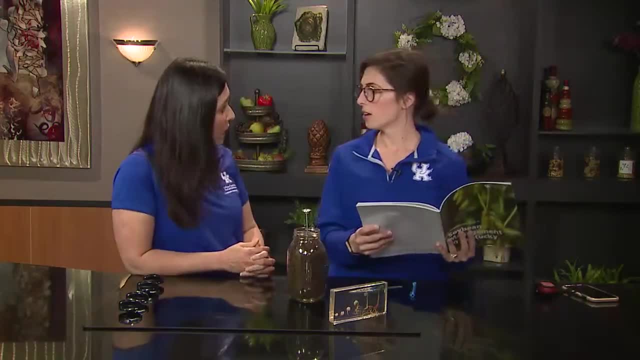 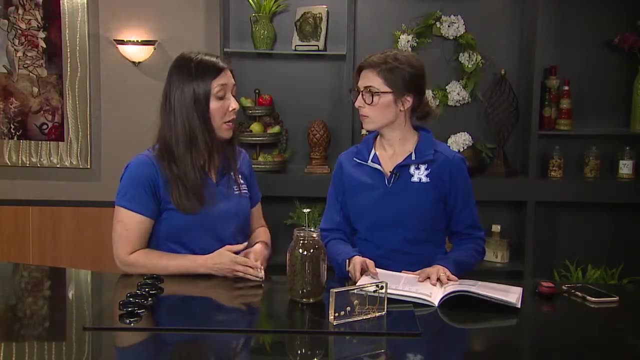 what the optimum date is. But Kentucky weather doesn't always play along with our dates, And so this is why this is so important, So that you can tell. I mean you know, some years we've still had snow on the ground, Or we get a. 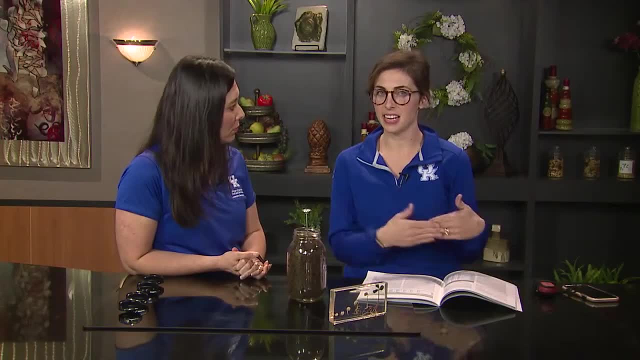 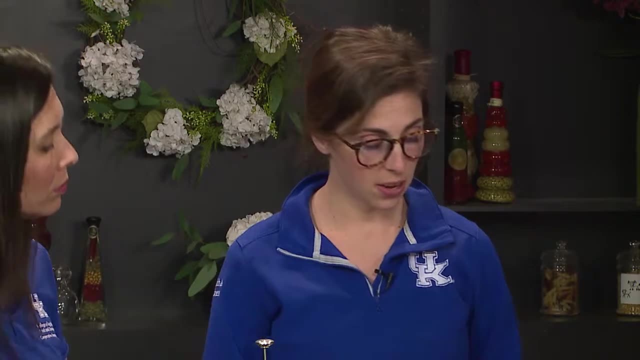 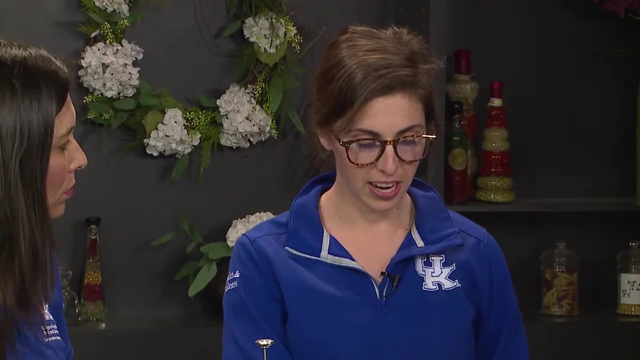 snow. you know it could warm up for several days and then it can drop back down. So they also have in this book- which I think is really cool- your probability of frost. So Henderson is listed on here, which is where I'm at. So 90% on April the 5th there's still a 90% chance that it's going. to frost And 90%. I mean, that's not like you know. that's a pretty high percentage. It's a pretty high percentage, But by April 20th we're down to 50% And by the 1st of May we're down to 10..